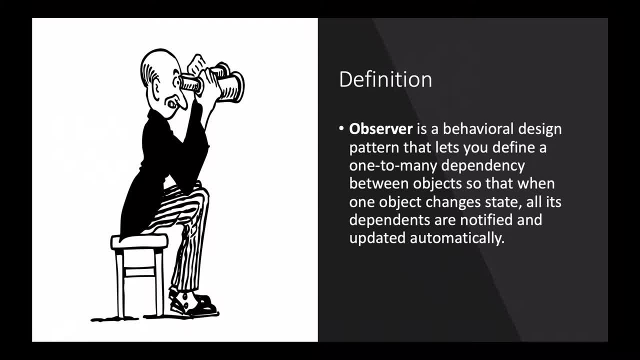 lets you define one to many dependency between objects, so that when one object changes state, all its dependents are notified and updated automatically. So this is the essence of this observer design pattern. To make this more clear, I would like to show you a little bit about the observer design pattern and how it works. So let's get started. So this is: 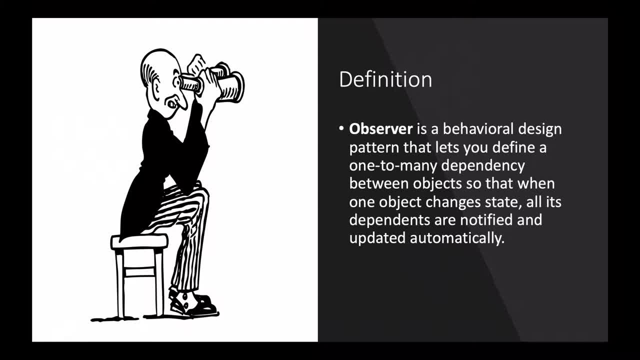 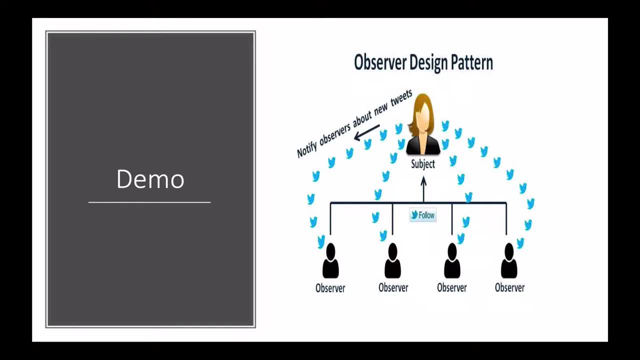 a diagram which represents this complete definition in one picture, So it will be very easy for you guys to understand this. So this is the diagram I was talking about and this actually describes the flow for this observer design pattern. So in observer design pattern we have two entities: The 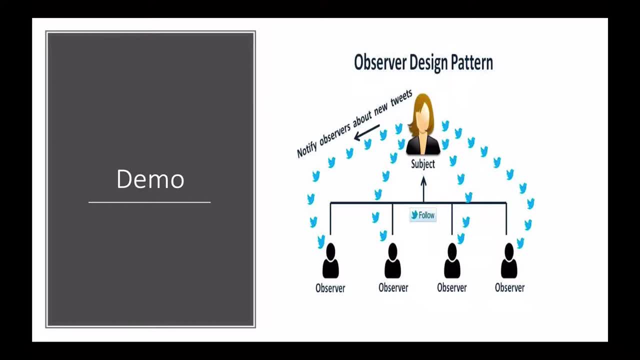 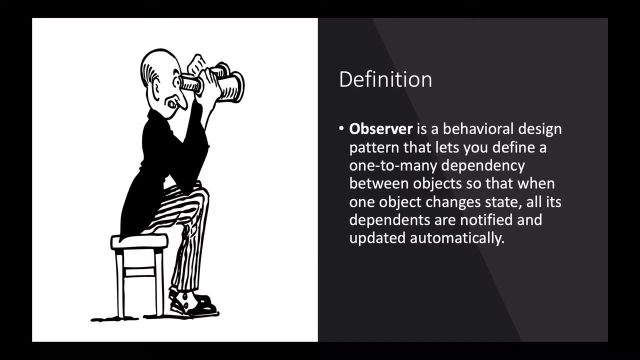 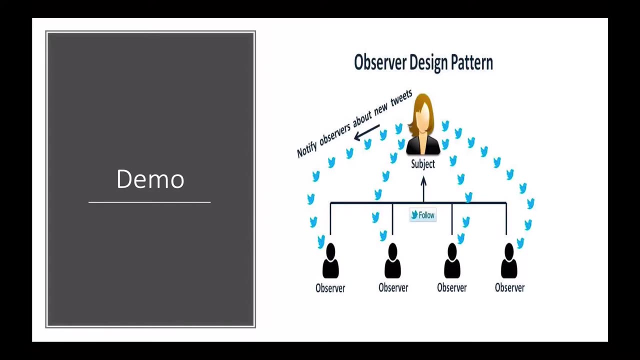 first entity is called the subject and second entity is the observer. and the idea behind this observer design pattern is it lets you define a one-to-many dependency. So, as you can see here in this diagram, we have a one-to-many dependency. Many observers are depending on one subject, So subject: 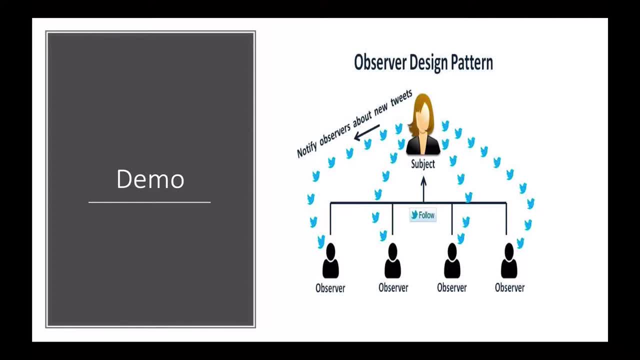 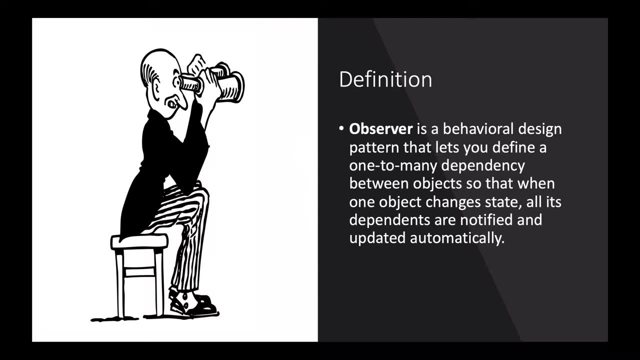 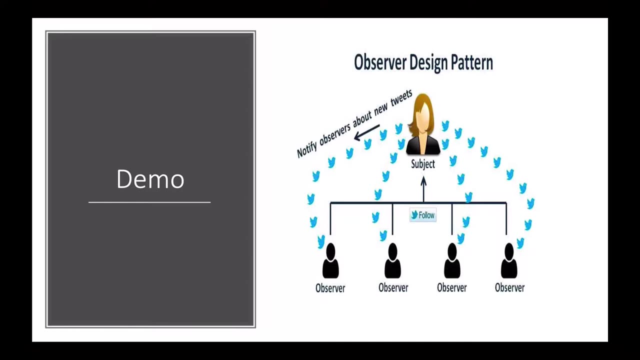 has a one-to-many dependency between subject and observer. The second part of the definition says that when one object changes state, all its dependents are notified and updated automatically. So here in this diagram the thing is, if the subject modifies its state, all its observers are going to observe that modified state and 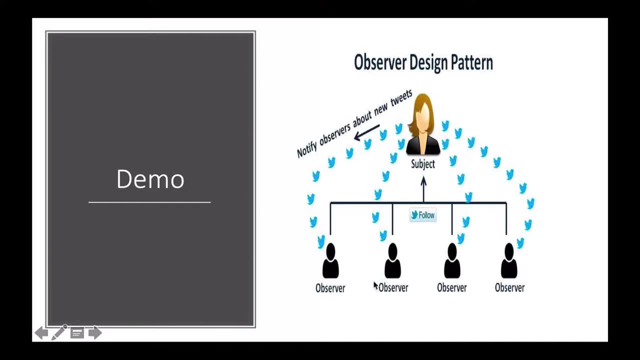 update themselves automatically whenever the subject changes its state. So this is the essence behind this observer design pattern: The observer is notified by the subject that there is a change in the state and observer can take necessary actions according to this. So you can imagine this. 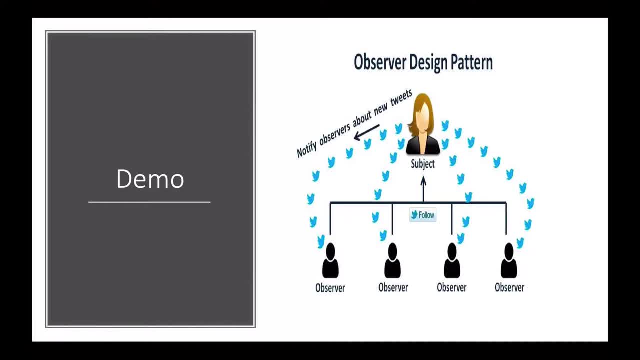 pattern in a whole lot of scenarios where there is one thing you want to observe and when, at the point, at the instant at which that thing changes, you want to do something. So whenever you are observing that this is the scenario you need, you should actually check the observer design pattern. 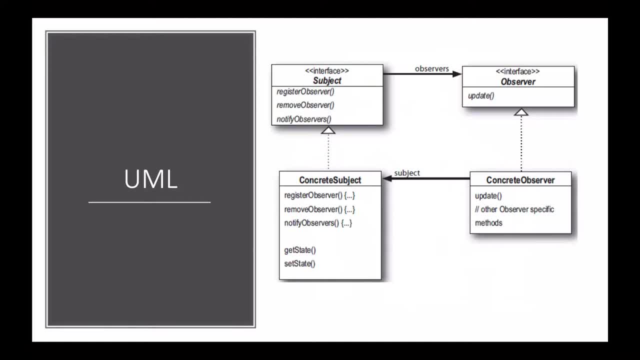 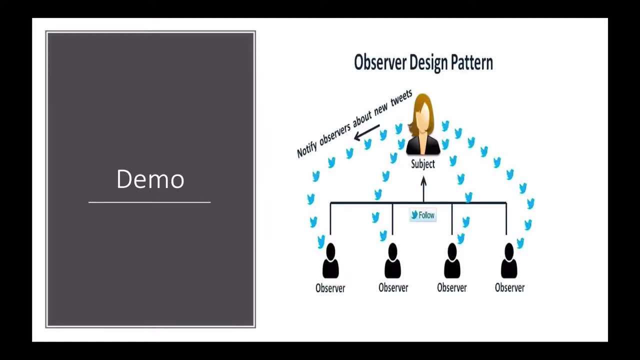 So let's take a look at the little UML diagram, which will demonstrate us more clearly how will we do this by code. So, as discussed, we have two entities here. the first entity, subject, and second entity is observer. In our UML diagram also, we have 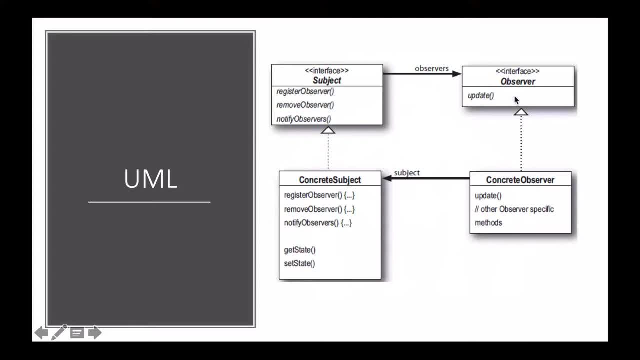 two entities, which is a subject and an observer. and subject has three methods, which is register observer, remove observer and notify observer. So this interface will be having three methods to qualify as a subject. Similarly, an observer will also have its update method. So what subject? 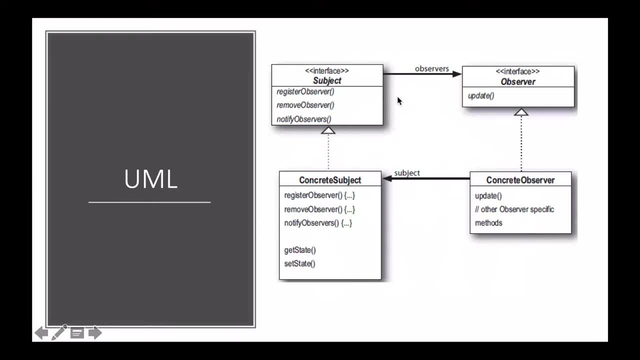 will do is, whenever there is an update in this subject's field, it will call update on its file. Now, since this is an interface, we need to actually build a concrete implementation for this interface which will provide implementation for all these abstract methods. We will create a concrete subject and a concrete observer and, as you can see, a subject has an 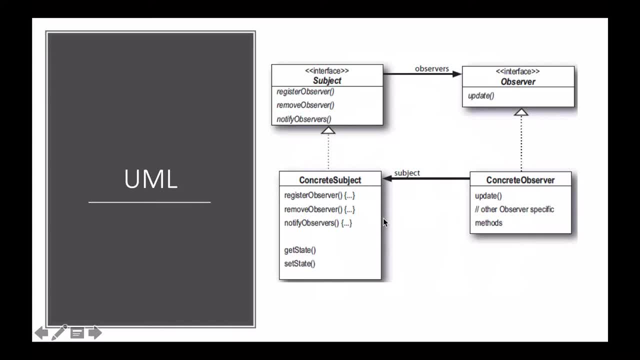 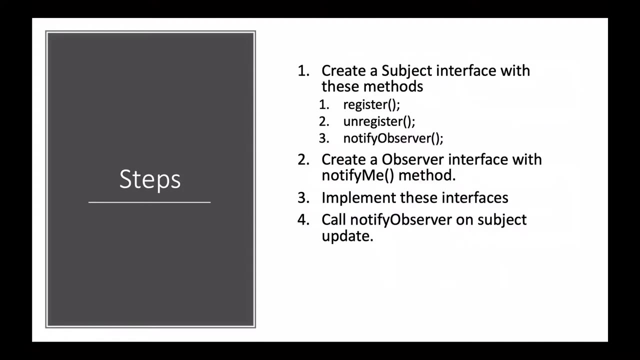 observer and an observer has a subject, and both of them implement from the corresponding interfaces. Now let's look at a set of steps which we need to define in order to actually code the pattern from scratch. so what we will be doing is: we will be creating, we will be. 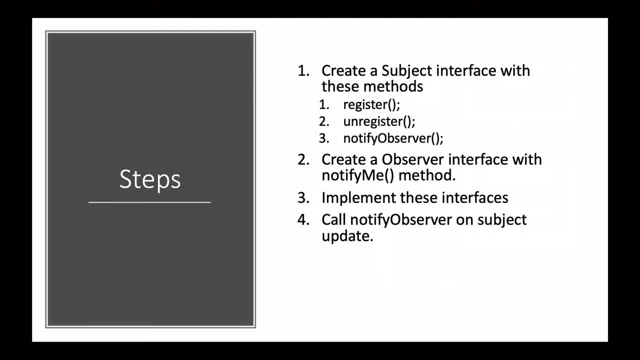 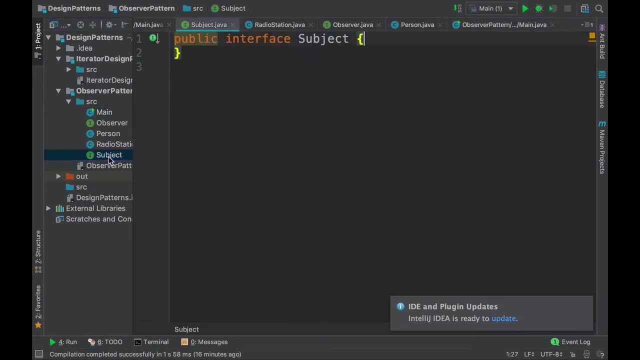 using the Java programming language to implement this, and the first step what we need to do is to create an interface, called subject, with these methods. let's go to our IDE and create a subject interface with these methods. so here we are in the ID and I have already created a class for this subject interface and 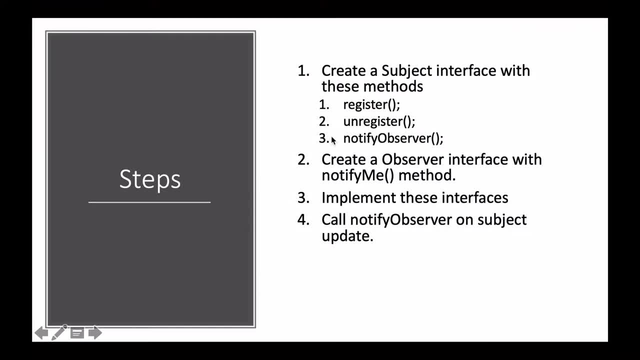 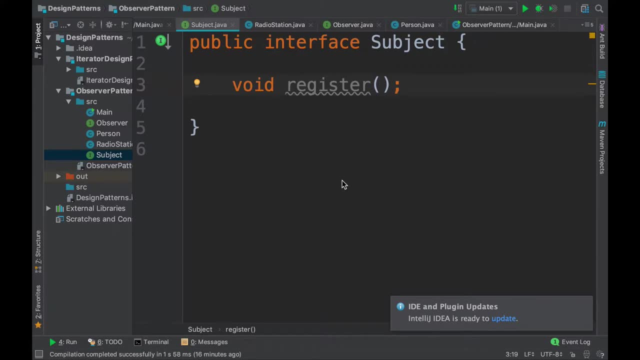 let's define these three methods. so the first method which we are going to define is the register method, so we will say void register. the second method is the unregister and the third method is the notify observer. now let's look at this method: signature one. so we want to register an observer to one subject. so 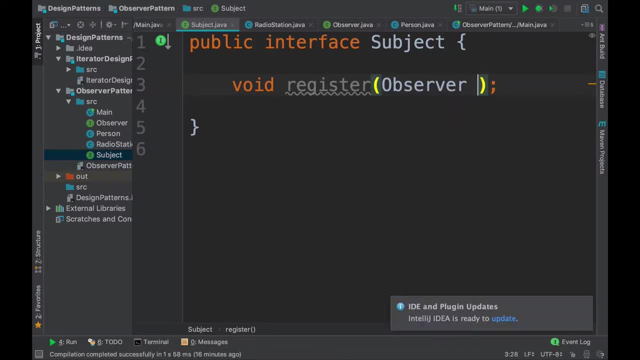 we need to take a observer class for this and this will take the observer and register itself. now, this unregister also. what we are going to do is we are going to create an unregistered method which will also take an observer and, given a reference to an observer, it will unregister this observer from the subject. now we need 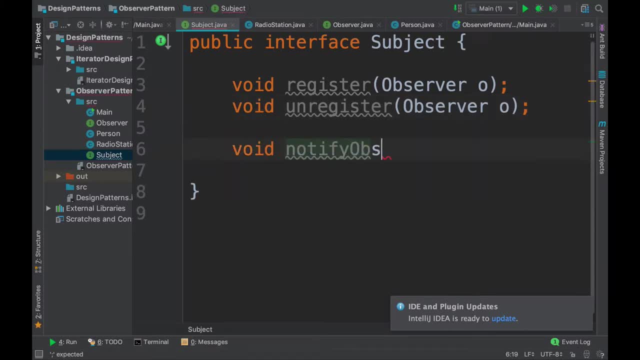 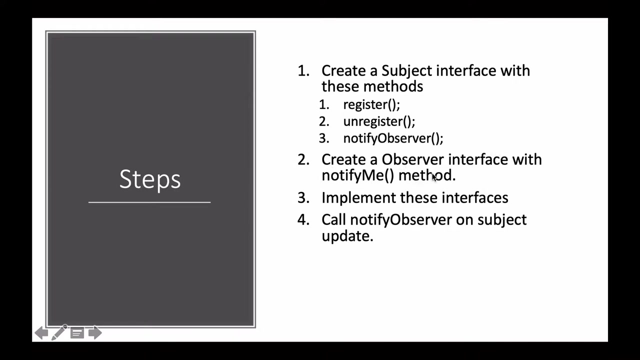 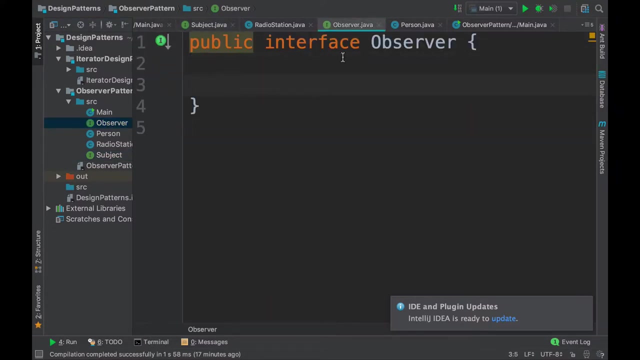 one more method, which is called notify observers, which we will be using to notify the observers, whatever are registered for this subject. let's go to the second method. the second point says that create observer interface with notify me method. so let's go to our observer interface. this is the observer interface and I have created this class. 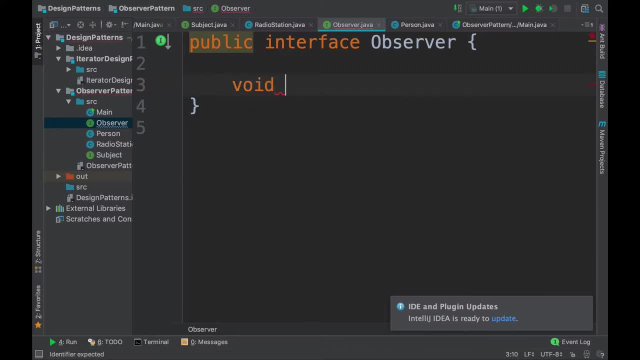 already. so let's go ahead and define the notify me method now, since we have implemented- sorry, define this notify me method. I have given an integer I argument, so I want to notify this observer with an integer I, so now we are done with the two steps in. the third step is to implement these. 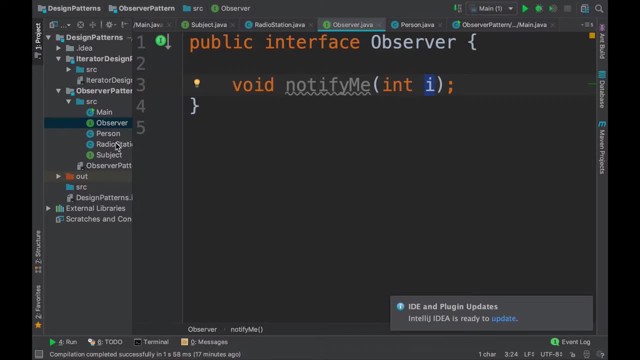 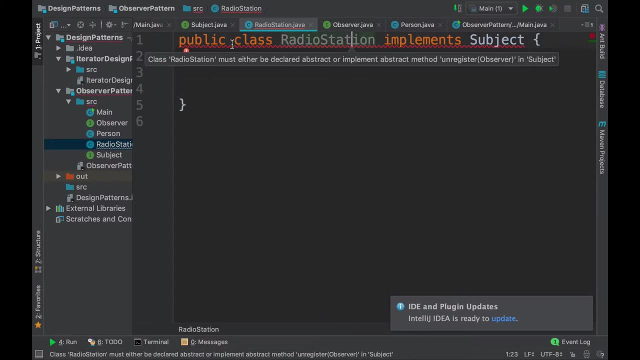 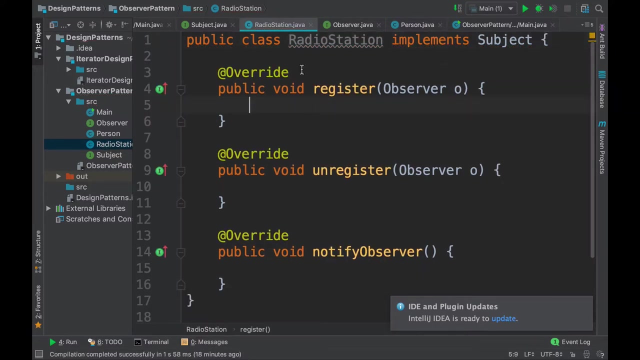 interfaces and provide the implementation for such strike methods. so let's go to our radio station class, which is the complete implementation for this subject. so what we will do here is we will implement this method, provided by our subject interface, and start coding. so the first thing we need here is a 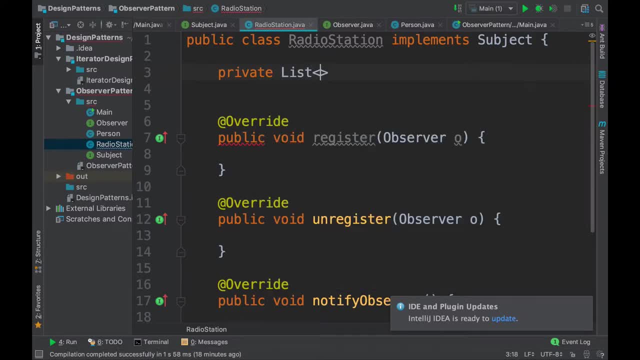 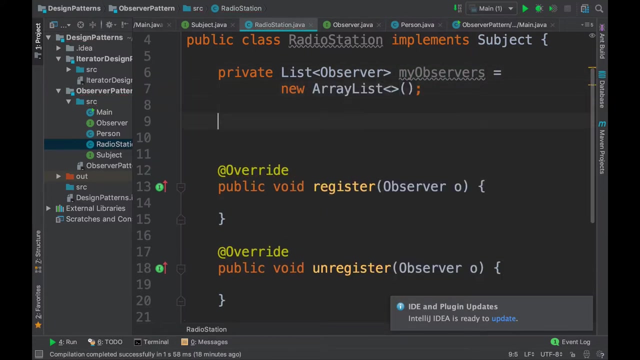 list of observers. so what we'll do first is WEARR: ugh, not again, sorry dude. I will say this next time: content: datasetiday- whatever will create is list of observer and we will call this my observers and we'll say new, add a list of observers. so now we have this list of observers and the 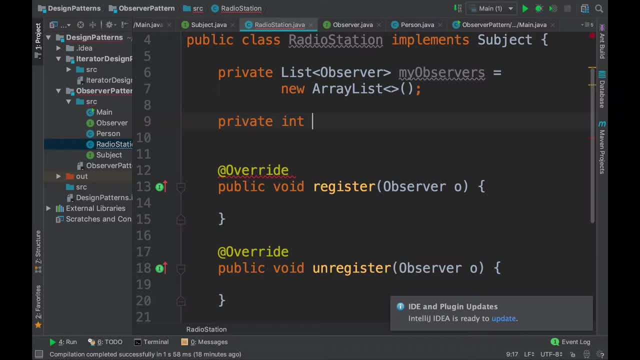 second thing I want to do here is create a variable which we will be updating to be so that the observers can be notified. so this is the variable. let's say, this is a golden number for a lottery ticket and this is 2, so all the observers will. 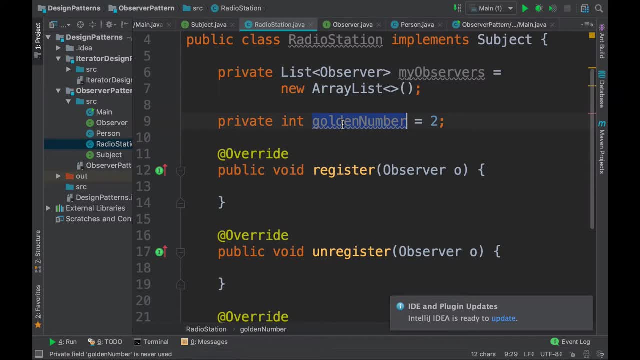 be registering to this subject and will be wanting to be notified about this golden number. alright, so the golden number is 2 now and whenever there is an update in this golden number, what we are going to do is we are going to notify all the observers- in my observers, so- whenever there is a register observer. 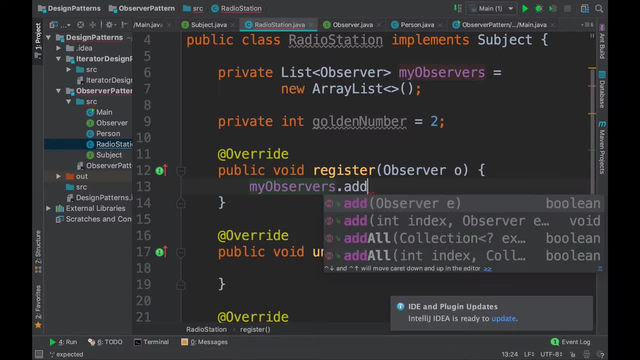 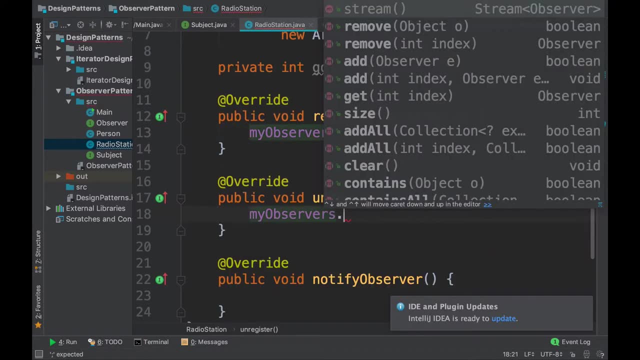 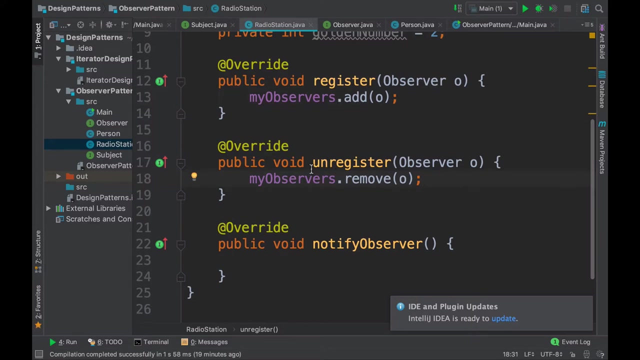 call. what we will do is we will take our my observers and add this observer to our my observer list. similarly, when we have an unregistered observer, we will call my observer and remove it from our observer list. so this is how we'll implement the register and unregister method. you could add your own logic for filtering and. 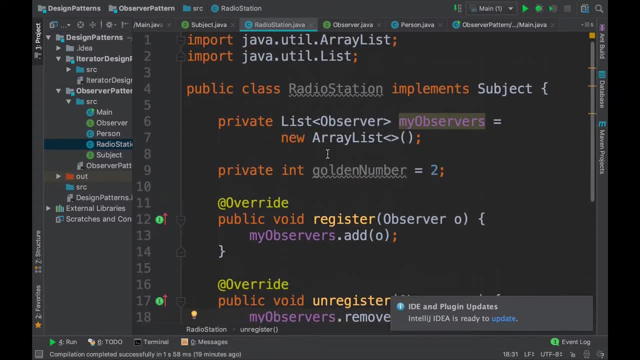 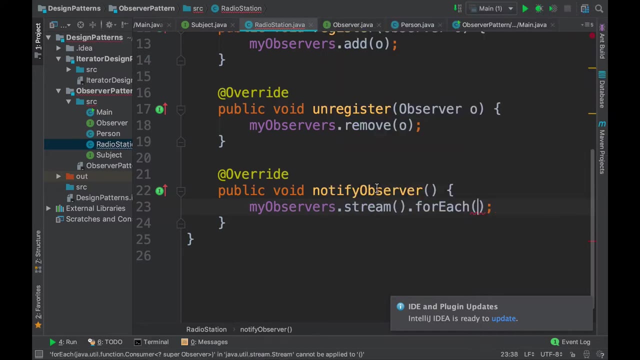 doing all those kinds of stuff. so this is a very simple example how we can implement this observer design pattern. now, regarding this notify observer, what we are going to do is, for each observer we want to notify itself, so my observer stop stream and we'll say: for each observer we want to notify itself, so what we'll? 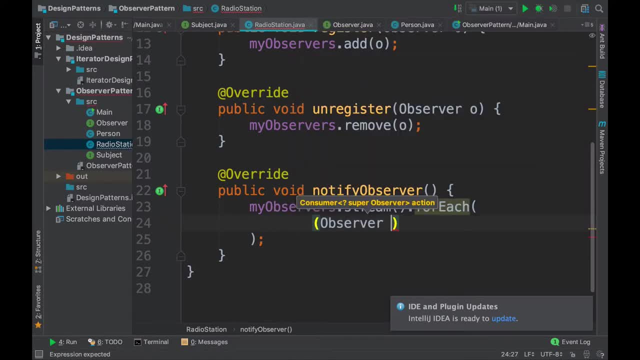 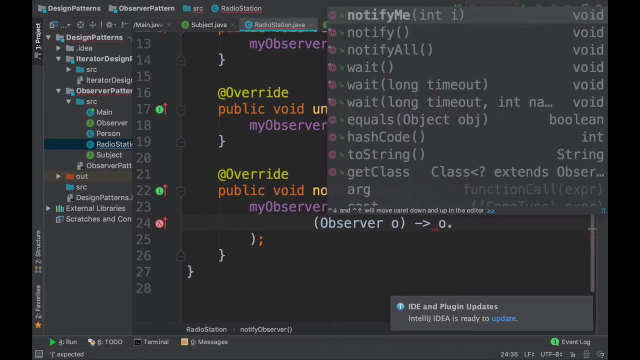 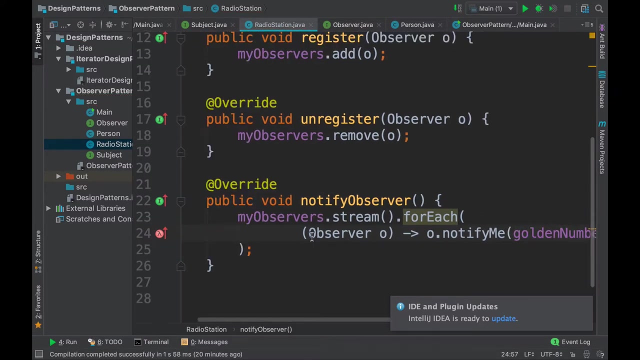 do here is we create a lambda function which takes our observer oh, and we'll call the notify me method on that and we will pass the golden number here, so whenever there is an update in the golden number. what we are going to do is we need a way to identify, notify all these observers. all right, so 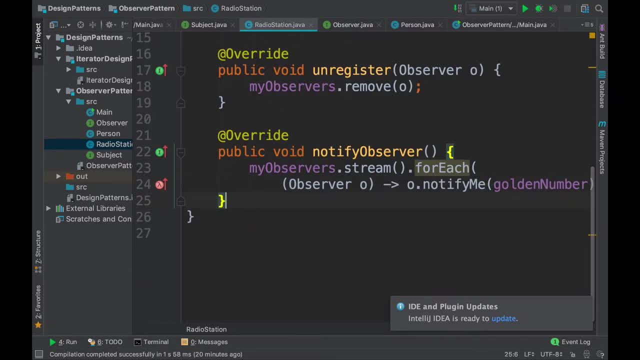 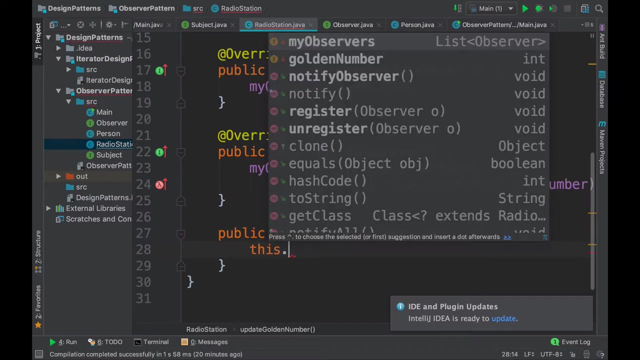 now this subject interface is ready, we need to add one more matter: to actually update the golden number. so let's add a method to update the golden number. we say update, called n number and we take a new golden number which is in tie and we say this dot golden number is equal to I. so now we are done with implementing the 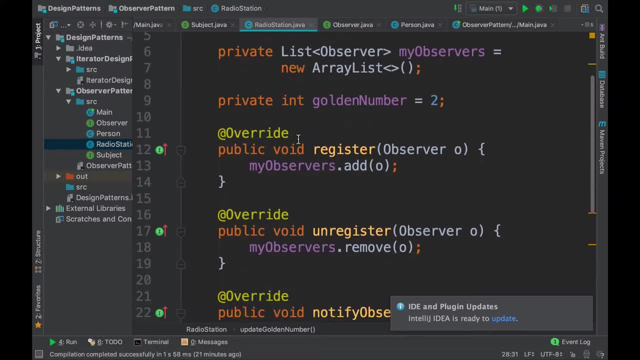 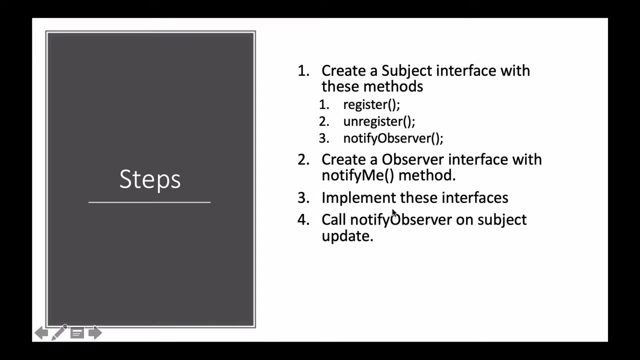 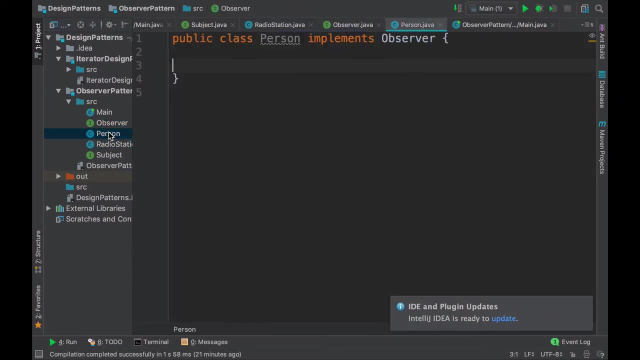 radio station class and we have implemented all these methods from the subject interphase. next step says: implement this interface. so now the pending uh thing is to implement the observer interface. so let's go ahead and implement the observer interface. so now i have created a person class which implements the observer interface. so what i am going to do here is we add all this. 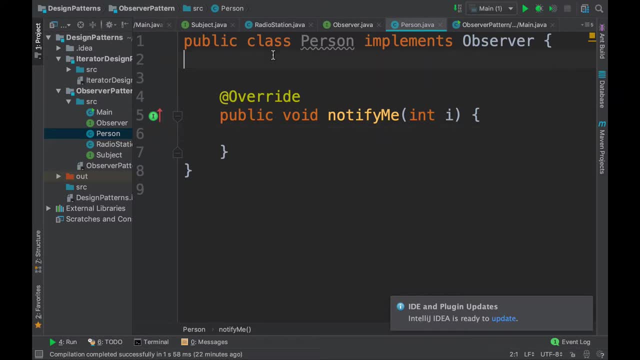 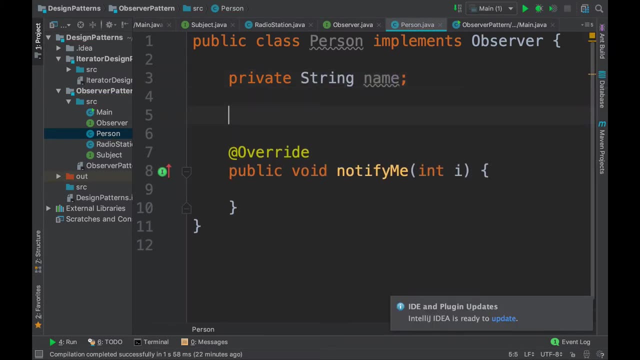 methods provided by the observer interface to this person class. so, apart from this, i would like to have a name for this person. so let's quickly go ahead and create a name for this person and, in the person constructor, let's take the name and set it. so now we have taken the name. 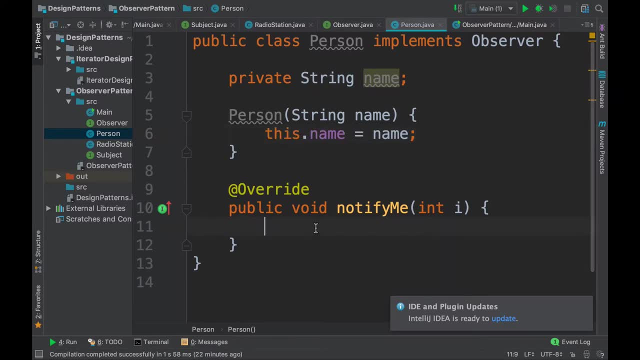 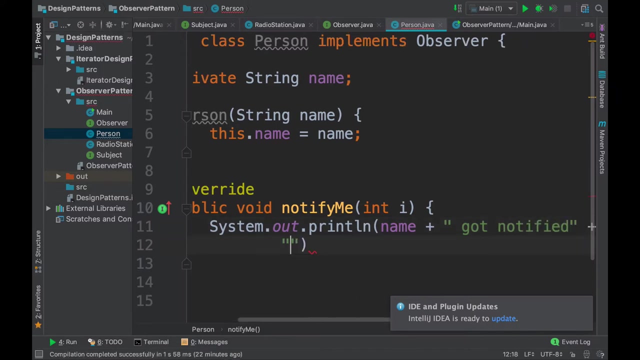 from the person constructor and setting it here in the notify me method. whenever a person is notified, what i want to do is i want to call systemoutprintln and i want to say that name got notified. and after the notification i want that the person should say that he got the updated golden number. so he will say: 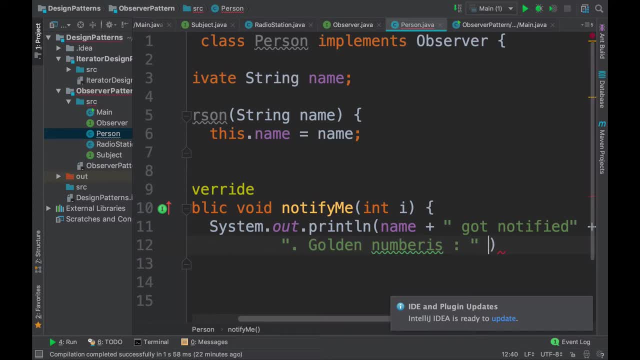 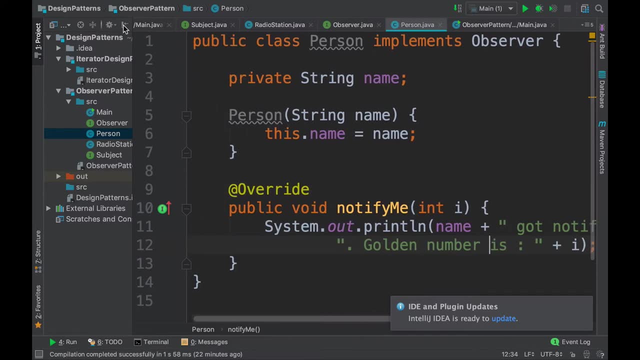 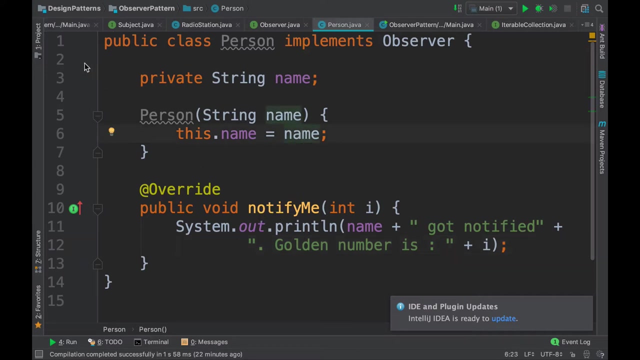 golden number is and he will display the golden number. so whenever a person is getting updated, he will say that he got the golden number and he got notified. so this is how the flow will look like. so now let's go to the main method, because that's the only thing we want to implement now, because we are 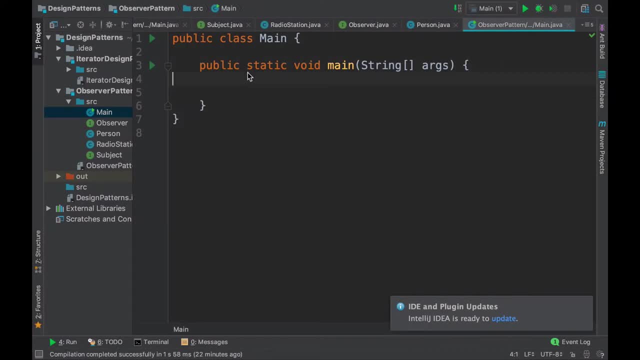 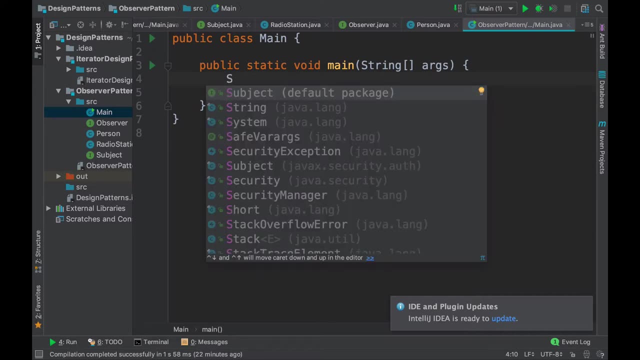 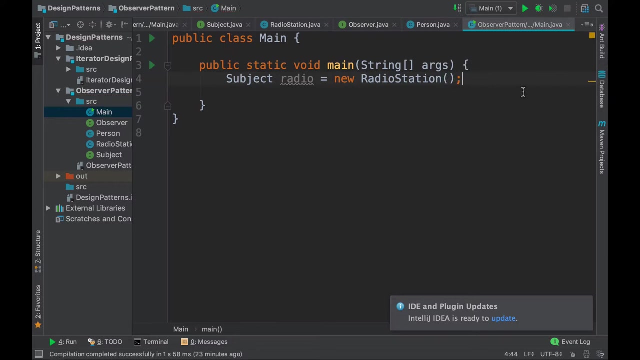 done with all these three steps. so we'll go to the main method and quickly, uh, construct a subject. so let's go to the. so let's quickly create a subject. so we'll say: subject: radio is new radio station, all right, and this does not take anything in the constructor. so we'll leave it like. 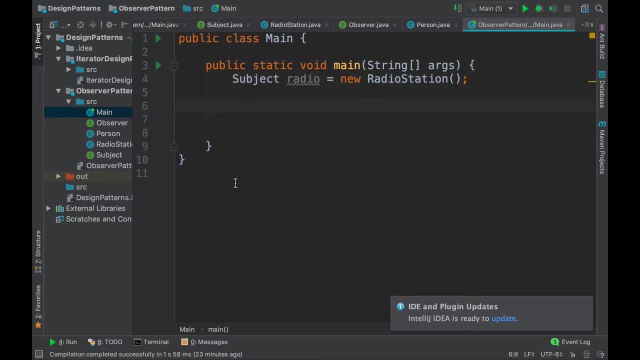 that and similarly, we want to create some observers. so we'll say: observer obi-wan is equal to new observer- sorry, let me undo that observer- and i want to create an observer with name black. so this is how i'm going to create some observers: let me create four observers and 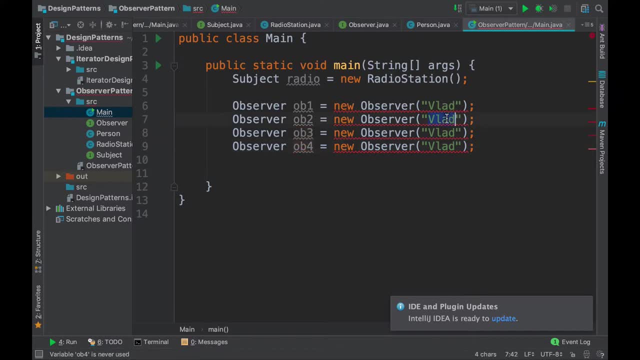 i'll name it observer one, two, three and four, and i'll simply change the name over here. so vlad, nico, roman and foston. so these are my four observers, and i have to make this person because i cannot create a instance of a interface. so let's go ahead and do it so now we have one radio station and 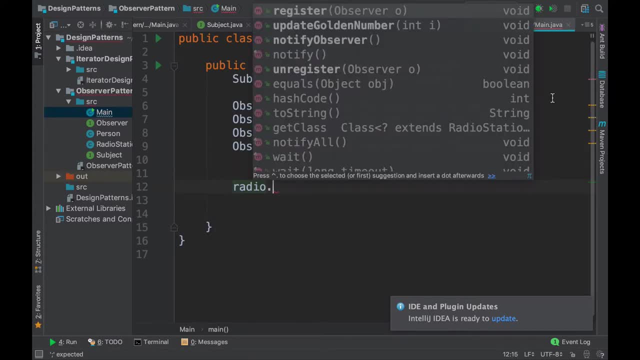 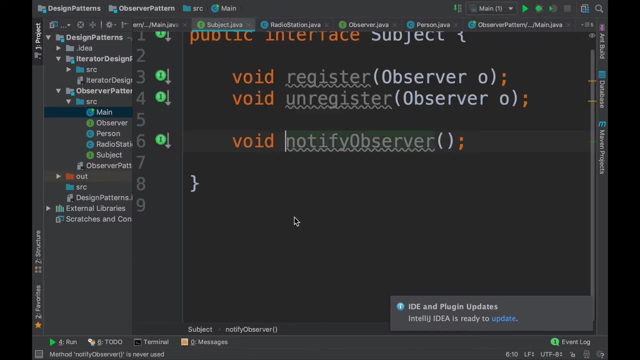 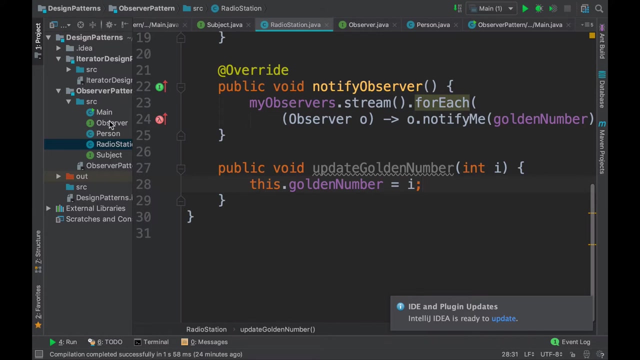 four observers, so let's try to uh notify observer. okay, so in the notify observer inside the radio station, what we have done is, for each observer, we are going to create a new observer and we are going to create a new observer for each observer. we are calling the notify me method. but now i just know. 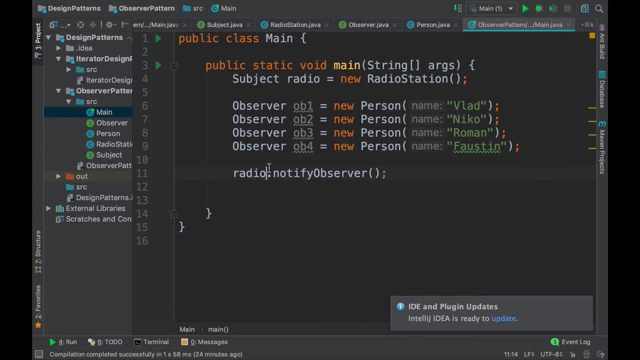 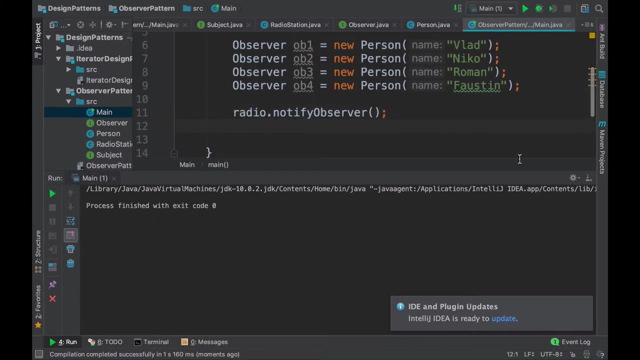 right now, that there are no observers right now. so if we try to run this code, we will see nothing. so let's go ahead and try to run this code and, as you can see, we are not seeing anything because we have not registered any observers yet. so now let's go ahead and 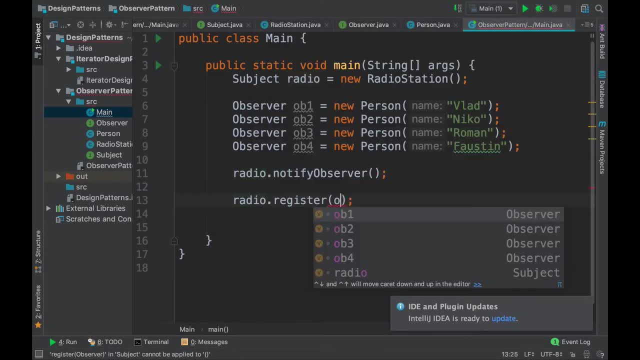 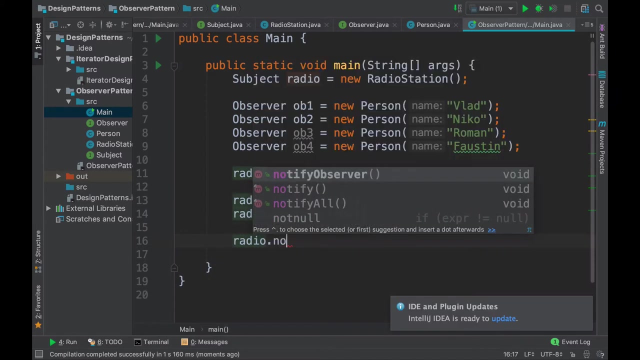 register some observers. so let's register observer 1, which is vlad, and also register observer 2, which is nico. so now let's try to again do a notify observer. so this time vlad and nico should be notified with the golden number, which is 2 by default. so let's run this program. 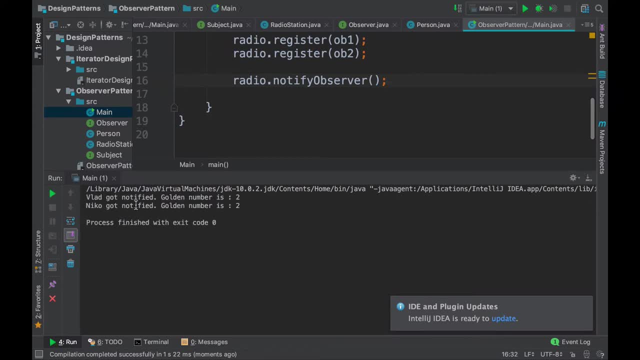 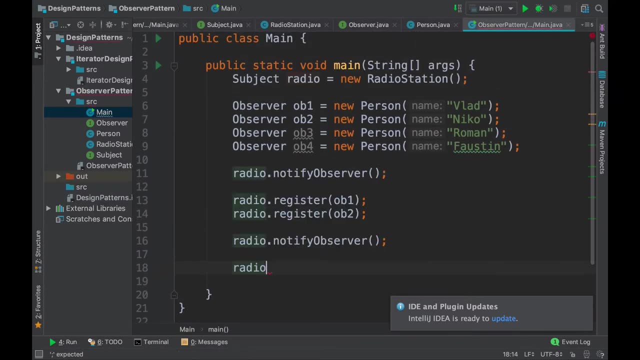 and you can see that vlad is saying that vlad got notified and nico is saying that nico got notified, and the golden number is 2 for both of them. now let's go ahead and add one more observer to this observer list, so we are going to register ob3. 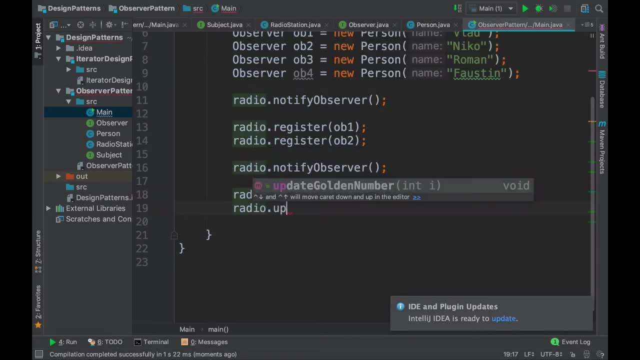 and also at the same time i'm going to modify. so i'm going to say: update golden number to 4 and this will notify all the registrer observers right now. so after this, there are three observers for this and this update should also update and notify all these. 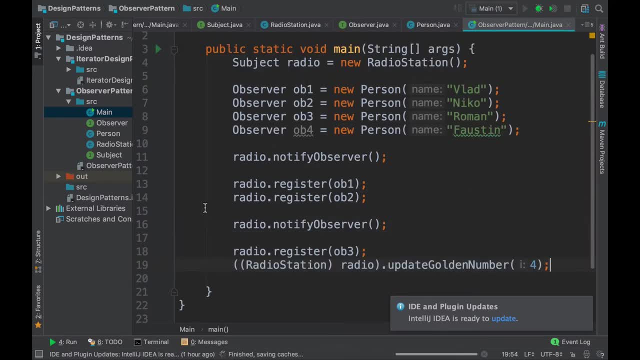 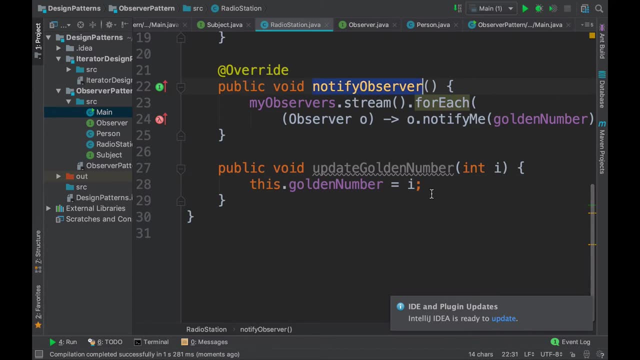 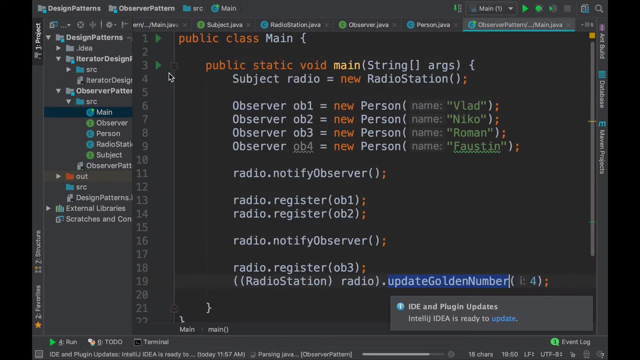 three observers. so let's now run this program and you will see that firstly. okay, so since i'm not calling the notify observers here, we are not seeing the results. so ahead here and call the notify observers also here, and now go to the main method and do a run. so now, yeah, you can see that after the update and adding a new, 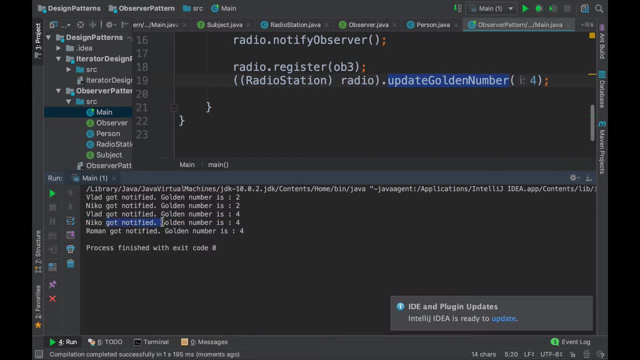 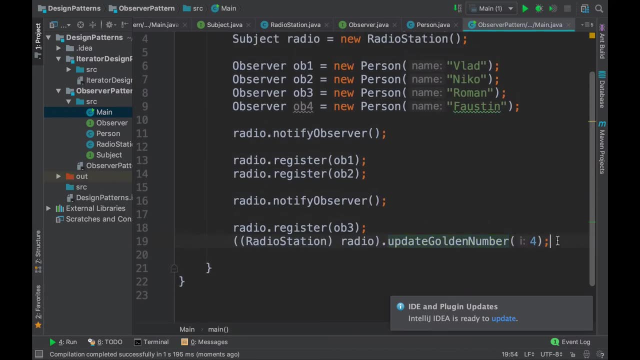 register whenever there is update. that is getting getting notified with the new number, nico is getting notified with the new number and Roman is also getting notified. now let's try and go ahead and start removing some of the observer. so let's unregister ob1 and let's add. 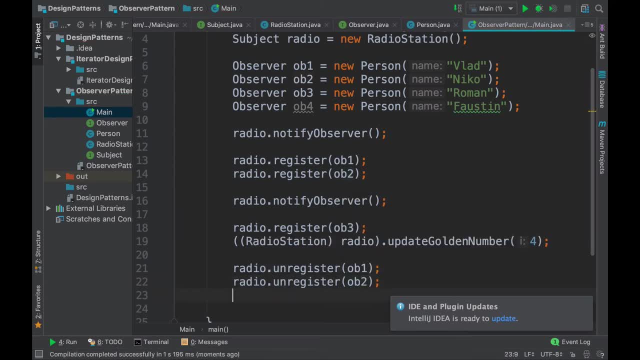 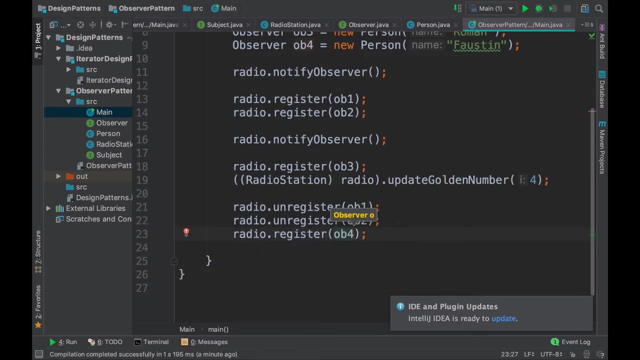 it's also unregister ob2, which is nico, and register fasten, which is ob4. and now we will say: radio dot 25, sorry, update, call the number. and whenever you are saying you radio don't update, call the number. now, this time we are going to.